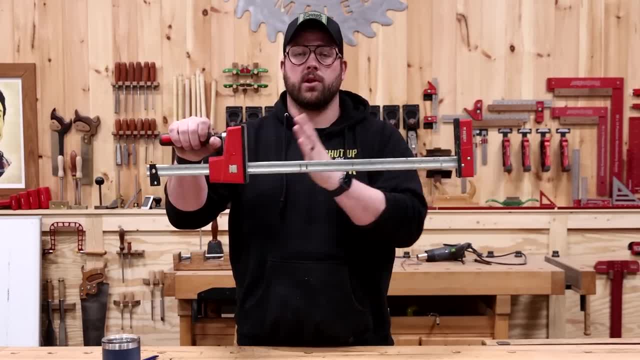 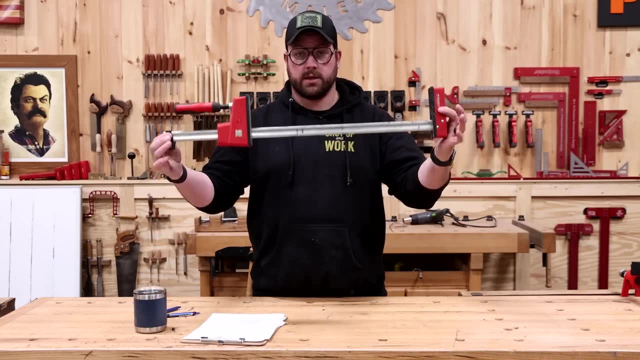 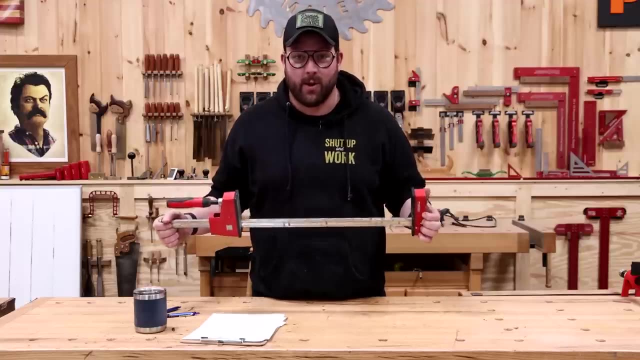 It's a parallel clamp and the intent here is to give you more uniform glue-ups whenever you're creating panels, whenever you're building stuff. Problem is this sucker right here. the single 24 inch K-Body Parallel Clamp Costs 40 bucks- Not that bad, but you definitely need more than one clamp to glue up a panel. 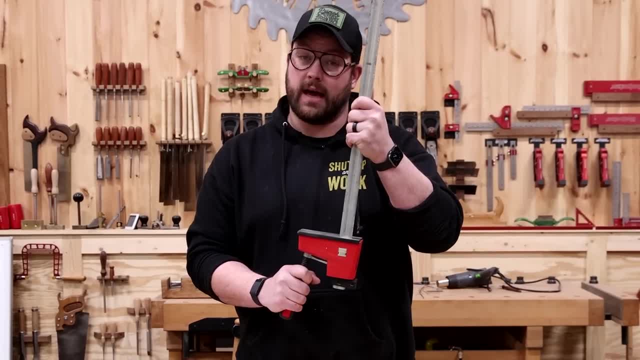 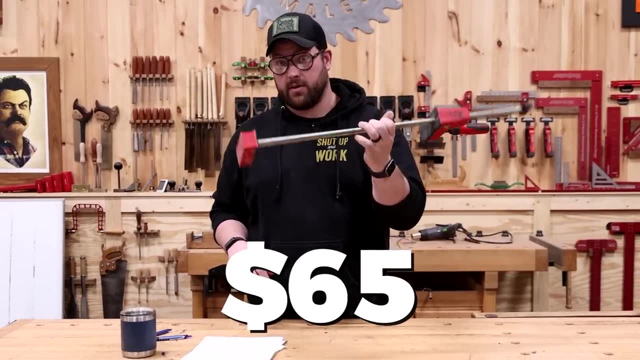 And then you also need clamps to be longer a lot of the time than just 24 inches To get into a 40 inch clamp. you're looking at $61 and the 50 inch clamp is $65. So this easily could become a very 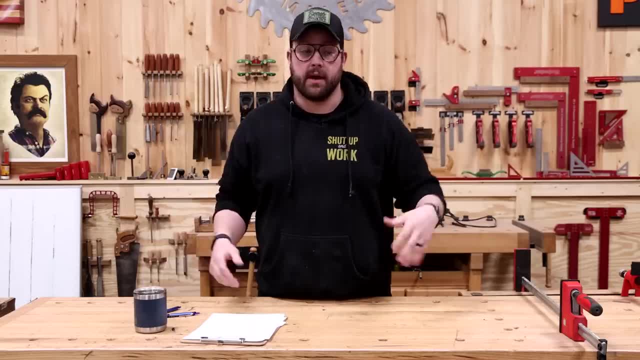 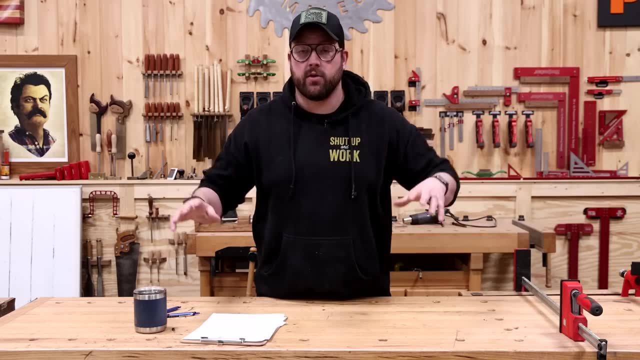 very expensive type of clamp to have in your shop. What I thought when I was a beginner was that these clamps were going to make my glue-ups way better because they're cooler looking and everybody's using them on YouTube, When in reality, if you go to professional shops, what you're finding much more often are these: This is a pipe. 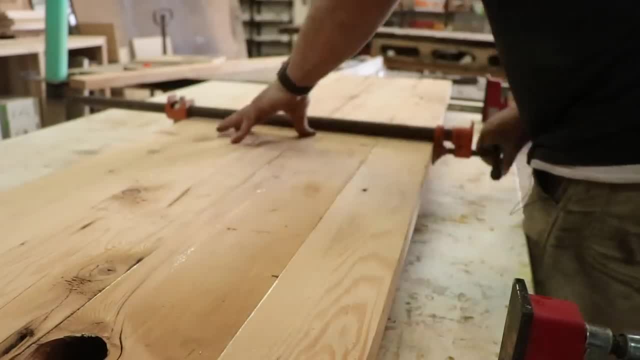 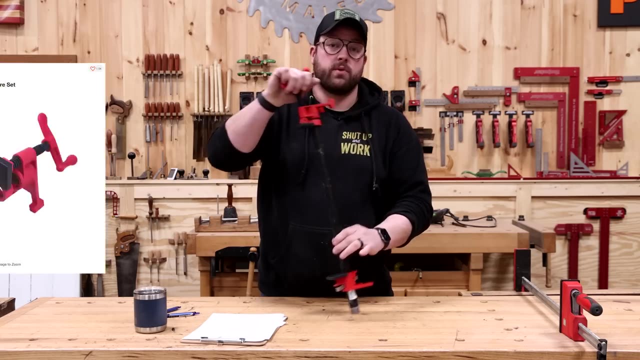 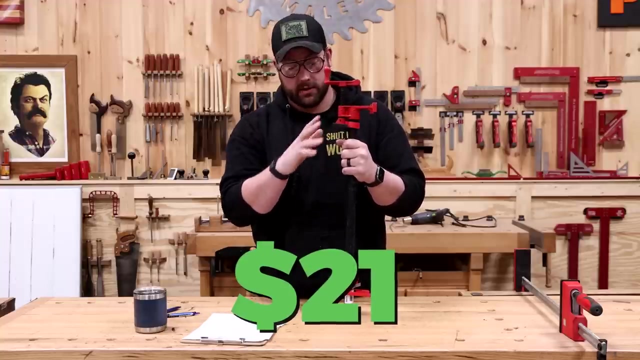 clamp. Pipe clamps are what I got started with and what I used primarily in my beginner woodworking journey. Few reasons for that. One one of these three quarter inch pipe clamp kits. if you want to go with the expensive one, this one's by Bessie, I think they cost you right around $21 for just. 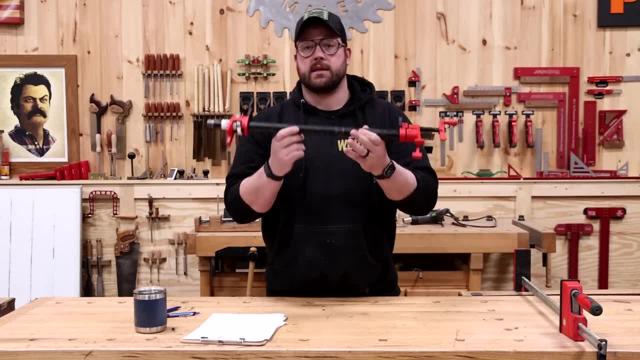 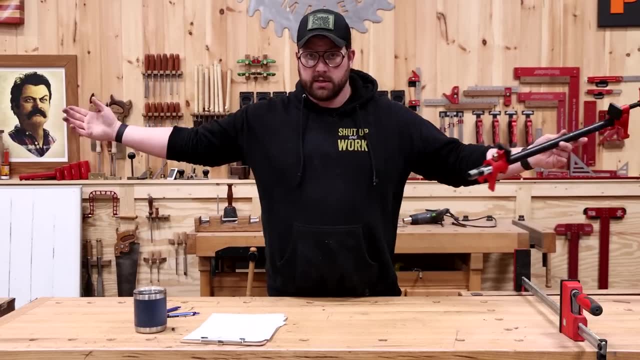 this clamp, So you're already at half the price. Now these can be used on three quarter inch black pieces. This piece of 24 inch costs about 15 bucks, but you can literally use as long as a pipe as you can find on these, which is amazing. You can also use couplers on the end of the pipe and thread a. 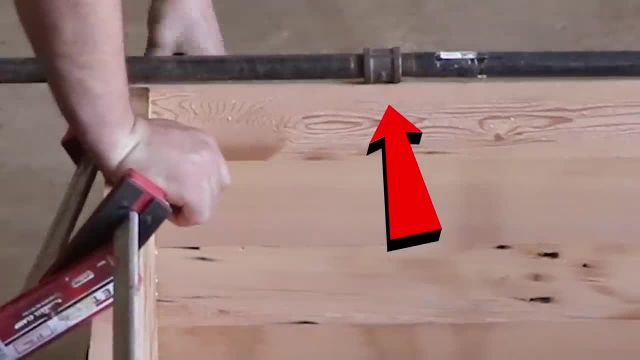 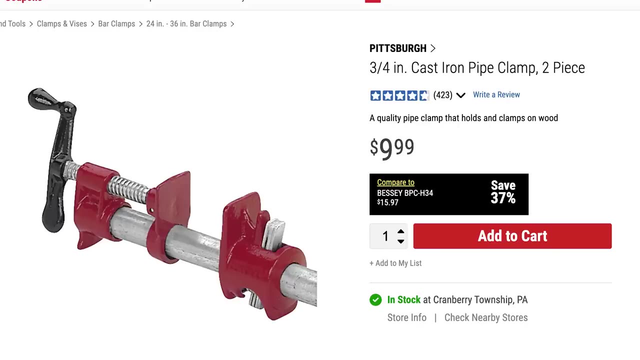 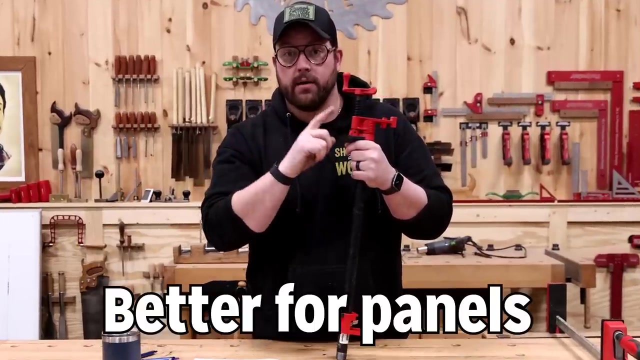 bunch of them together to give you really, really long clamps when needed. If you're cheap, like me, you can buy the same type of clamp at Harbor Freight for 10 bucks, So you're going to get into having more clamps at a more affordable price, And then, on top of it, I also think they're better. 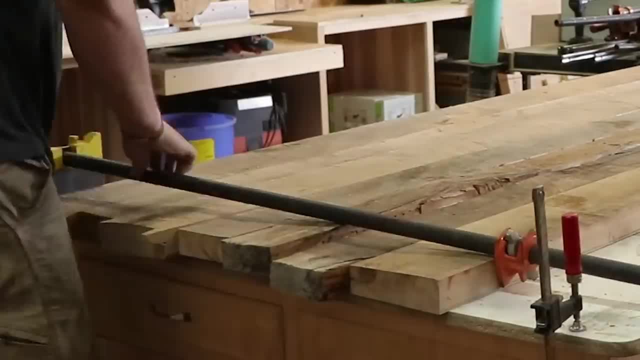 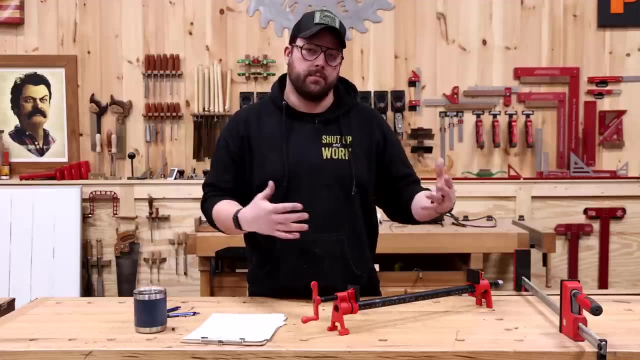 for panels. Why, you might ask. Well, in all my experience I've built a lot of big stuff And unless you have a great joiner planer setup, you're going to need clamping pressure to help you glue up good panels. And with 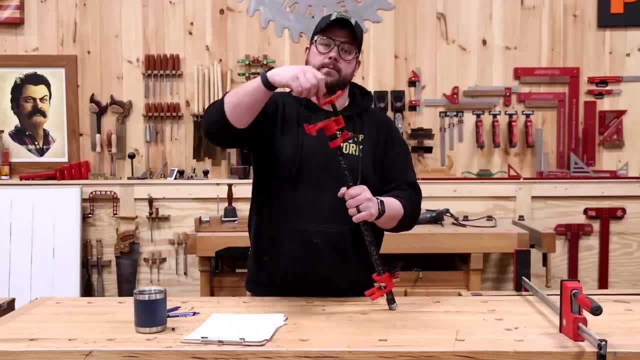 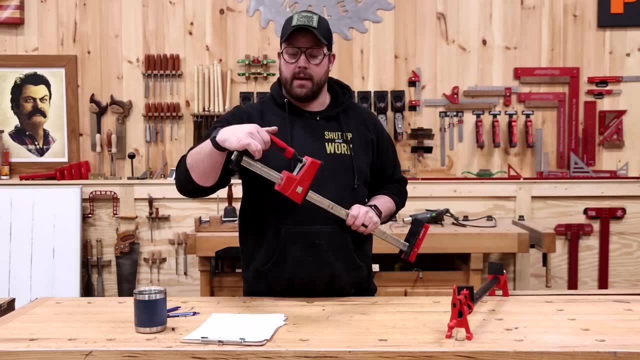 this type of a handle system that comes on a pipe clamp, you're going to get a lot more opportunity to put more pressure into your glue up than you are with the handle on the K-body or one of these Revo clamps. Now, all the pros and the guys that have super pristine tools that are really high end. 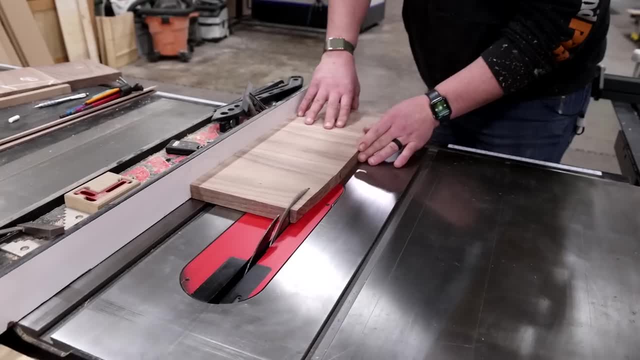 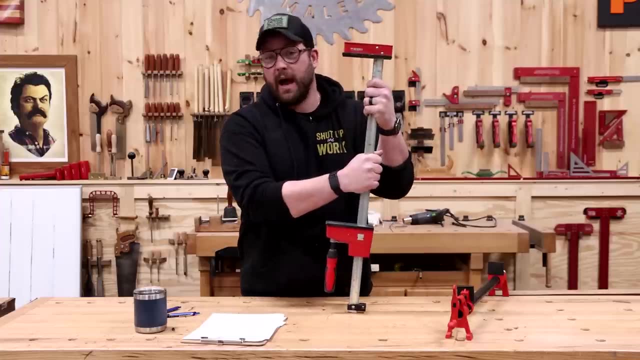 are going to get great glue joints right off of their joints, So you're going to have a lot more pressure on your joints than you are on your table saw. But I know as a beginner that's not always the case, And so what I found was, once I started investing in these, I was buying them on sale and I 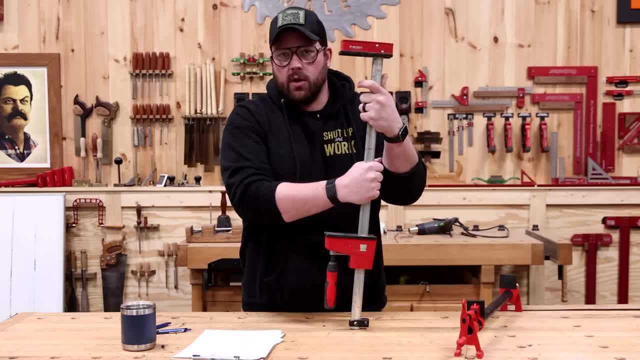 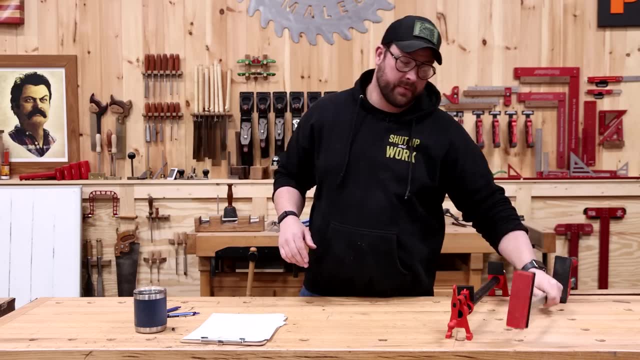 was stockpiling them, thinking they were going to make my glue ups better, And they just don't. You can't get a ton of pressure and they're not going to make your woodworking any better than what you can do with a pipe clamp. So first tool that I don't think any beginner should invest in early. 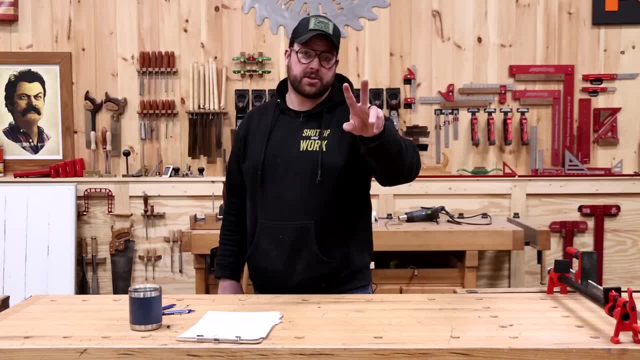 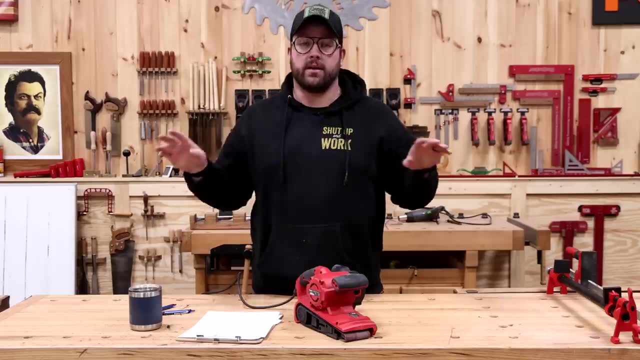 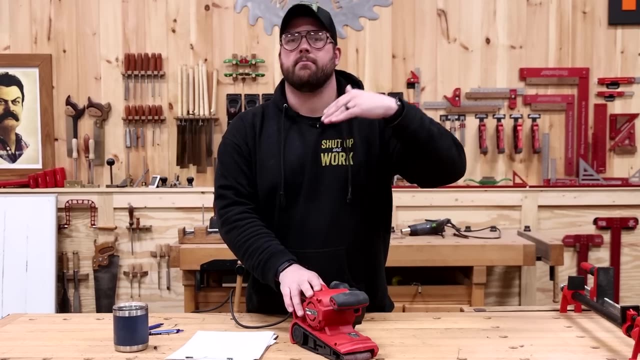 are going to be the parallel clamps. The number two tool that I don't think a beginner should invest their money on is going to be the handheld belt sander. First and foremost, I only know, like two woodworkers who are really good, that can use a belt sander in a way that doesn't actually make. 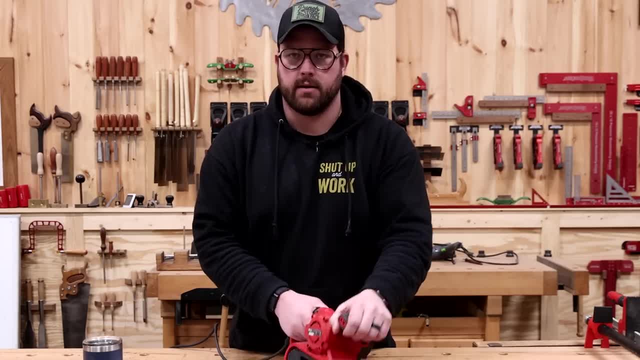 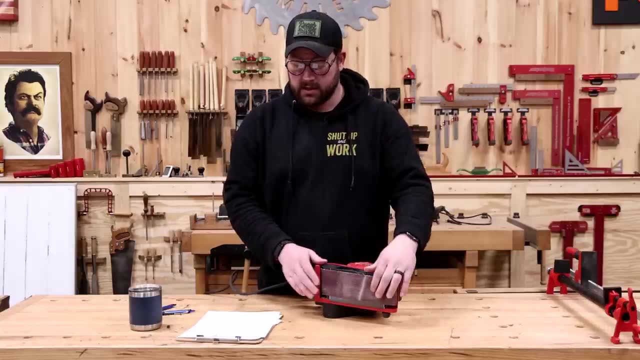 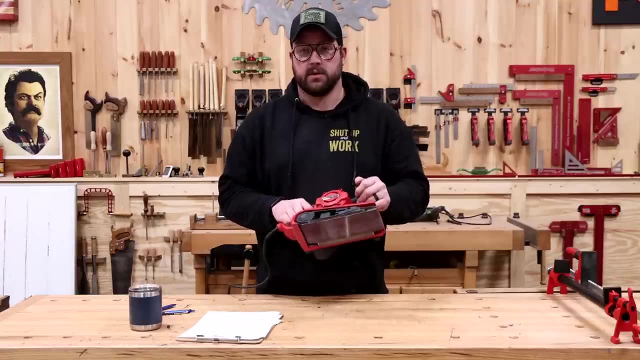 it more difficult than it does easy. The intent here is for large material removal with this tool, But when it comes to value and price, one of these suckers at Home Depot is going to run you like one hundred and sixty bucks, which is a lot for a sander, And this isn't that one. 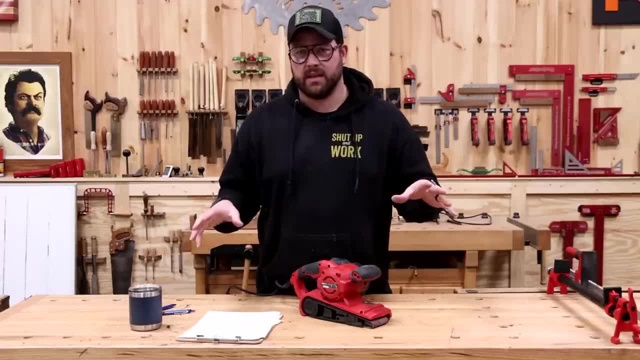 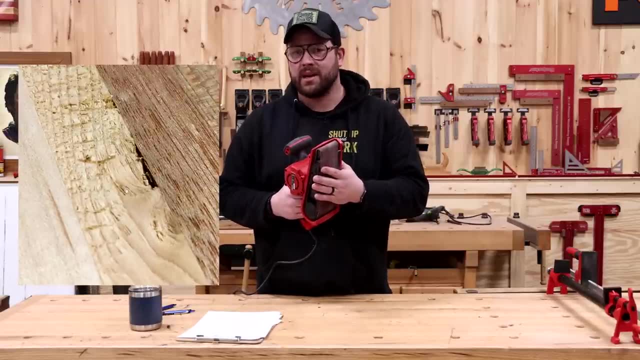 I'm not going to go into detail on this specifically, but between that and then the lack of utility in the sander, I just think it's a waste of money when it comes to using the tool. I've ran into gouging material a ton with a belt sander. 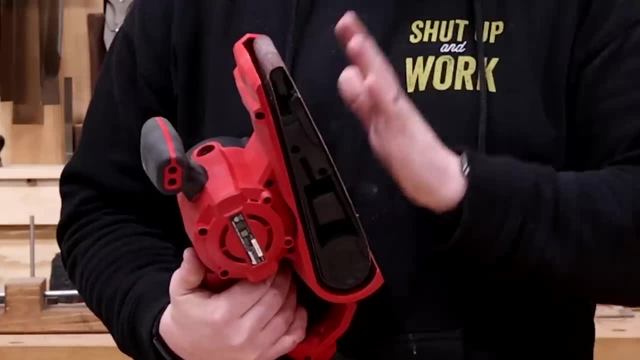 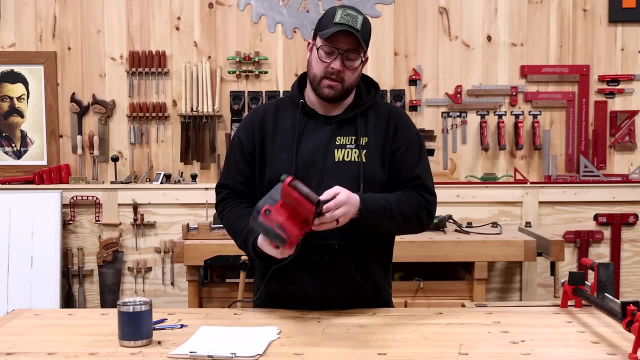 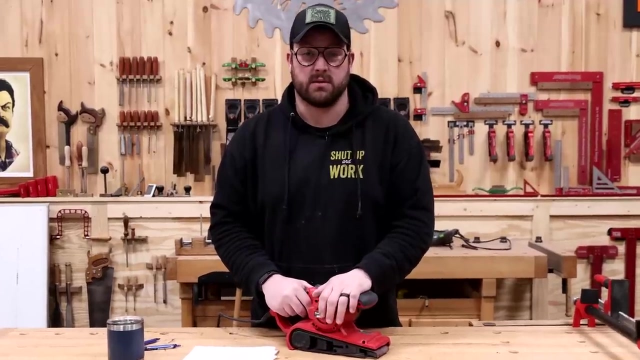 I've run into running into problems with the band, the band tension. Once it heats up it kind of expands, It falls off. Always having problems with that dust collection on it actually sucks because there's no way for dust to be collected inside of the belt itself And more or less like I just really realized that the tool is 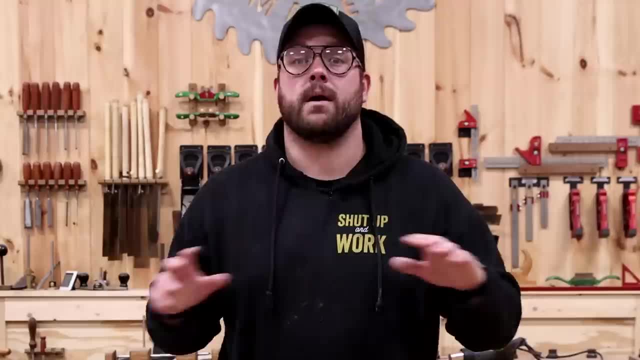 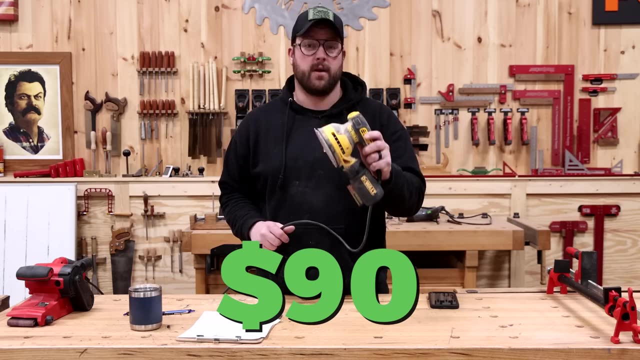 not what I needed it to be, And for the price you have much better options out there. So my advice is: for ninety bucks, go grab yourself one of these five inch random Orbit sanders from one of the box stores And it is a way, way, way better tool, in my opinion. You're going to get more usage out of it. 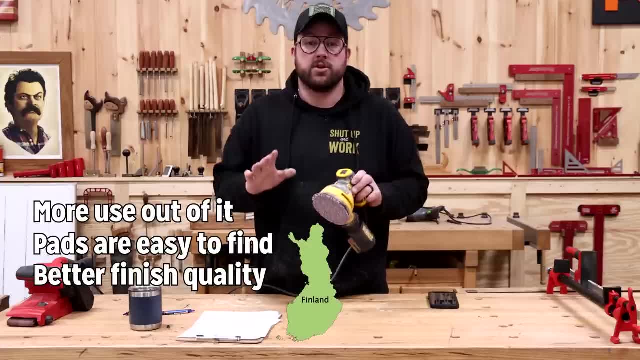 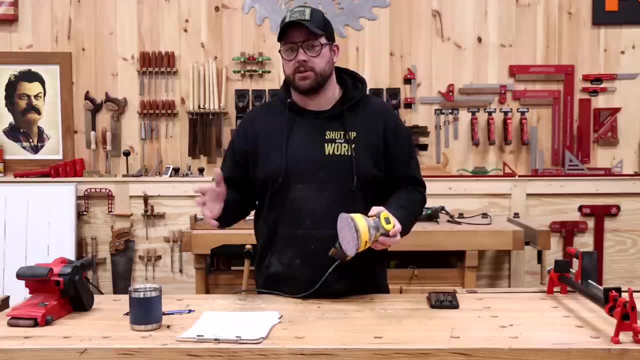 The pads are much easier to find. You're going to get a better finish quality as well. You can use this for a majority material removal as well as all the way up through your finishing And if you're looking for something a little more dainty. 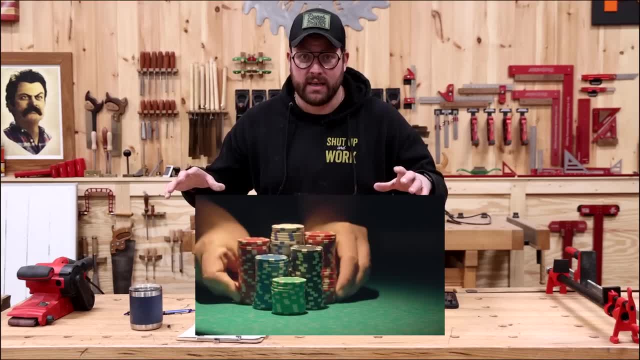 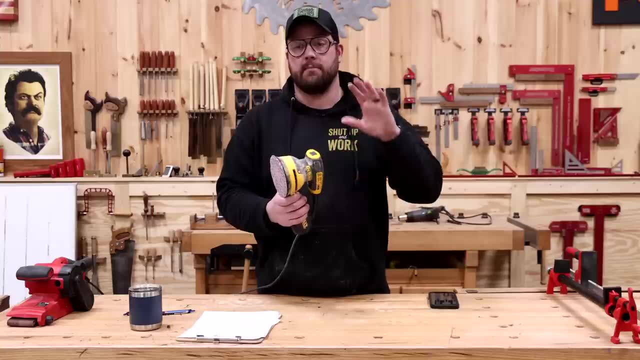 with your finishing for another seventy bucks, which is all in still cheaper than the belt sander. you can get one of the plate sanders that DeWalt also makes, And both of these, in my opinion, are a better option than a belt sander for a beginner. 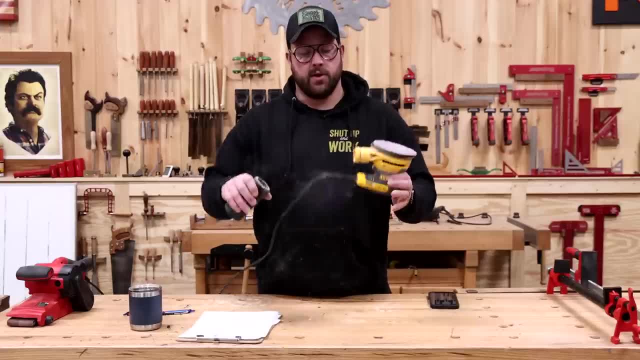 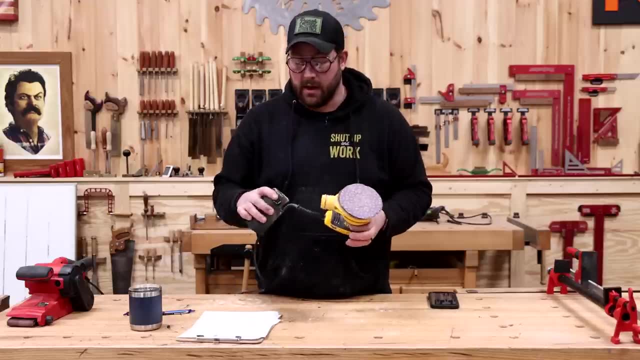 They're cheaper and they have more utility. Lastly, the newer models actually have the ability to have dust collection hooked up in one way or another, maybe with a little duct tape, maybe with a little 3D printed arm for your vacuum, But all in all, 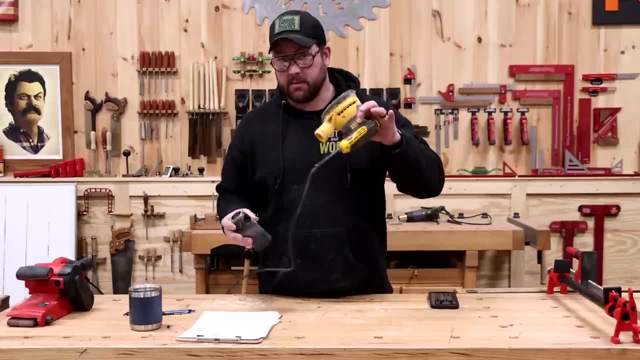 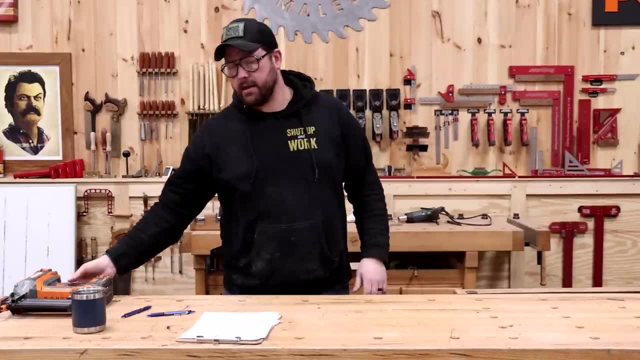 they're much better than what's going to happen with your belt sander And, in my opinion, just a much better and more valuable tool. Third tool that I don't think any beginner should get into or purchase is going to be one of these. 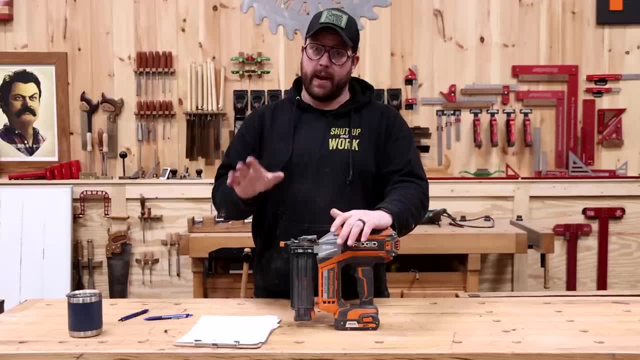 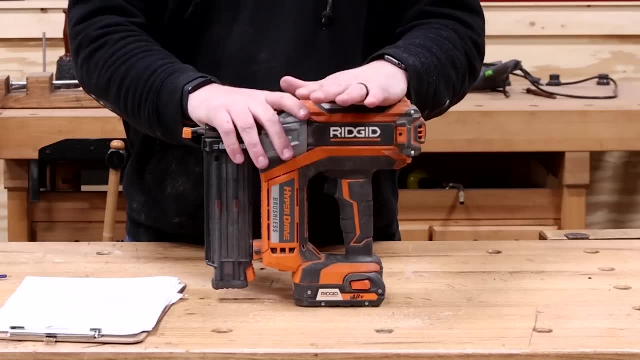 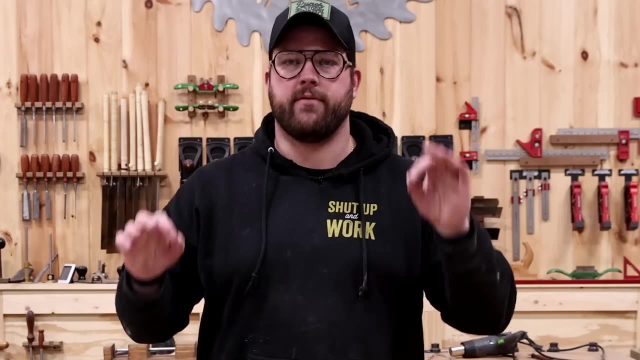 18-gauge cordless brad nailers. Now bear with me here. This is an incredibly popular DIY tool and I get it. It is versatile. You could take it pretty much anywhere. If you've got it on a specific battery platform, it can be an awesome tool. But I will say this: I have a better option. 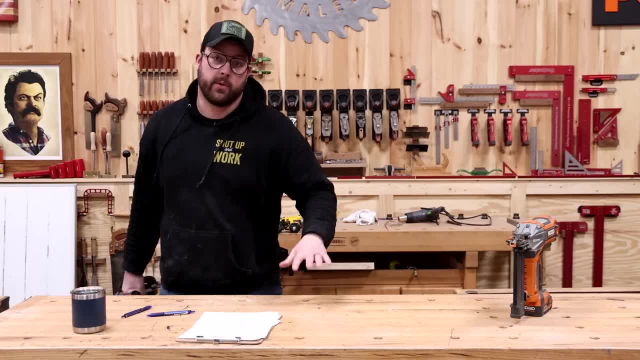 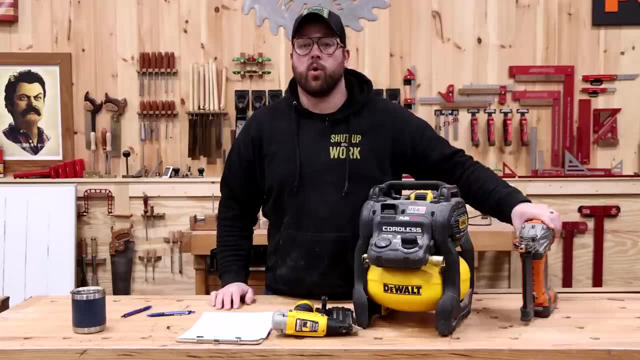 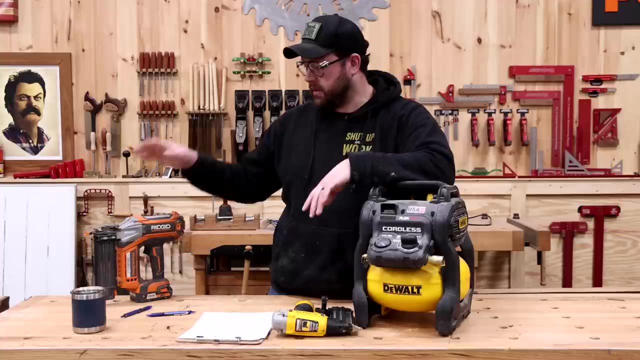 for you if you are just getting into the craft, And that option is going to be a cordless compressor and an 18-gauge nail gun. Now listen to me, The cordless nail gun itself is going to run you $250.. They're pretty pricey and as they should be. You can get them with and without a battery. 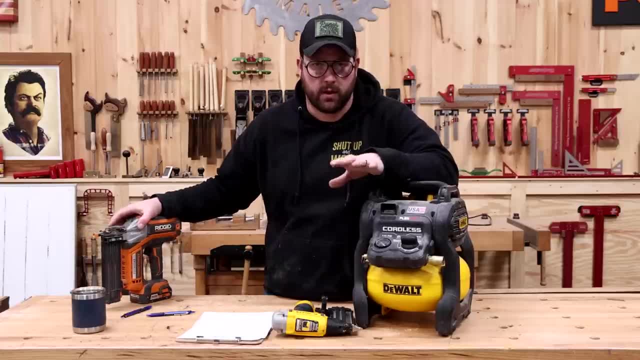 and I think RIDGID and Ryobi are making two of the most popular ones there are. If you're on those battery platforms, you can buy them without. They're probably a little bit cheaper, But with that comes the fact that this is a good tool. 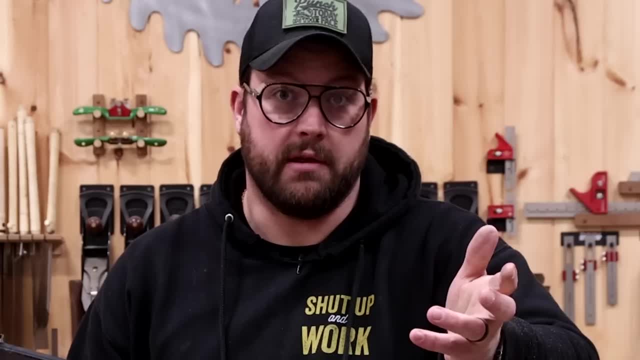 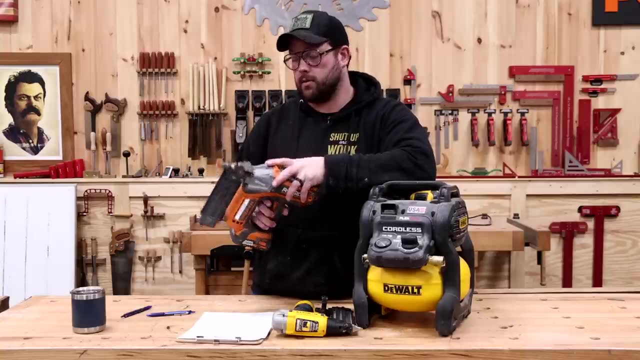 This is a one-trick pony. You can only nail with it more or less right, And you can only nail 18-gauge brad nails. So for $250, you can do one thing with this tool. For $219, you can get into this compressor. 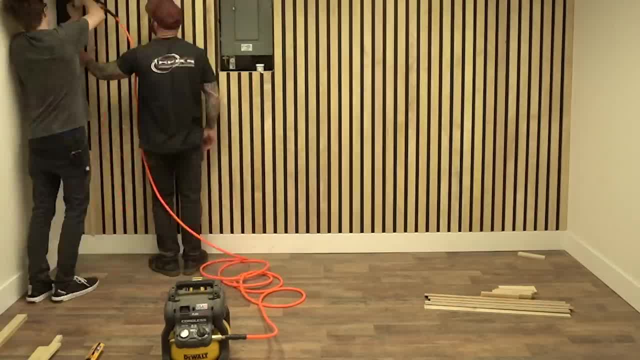 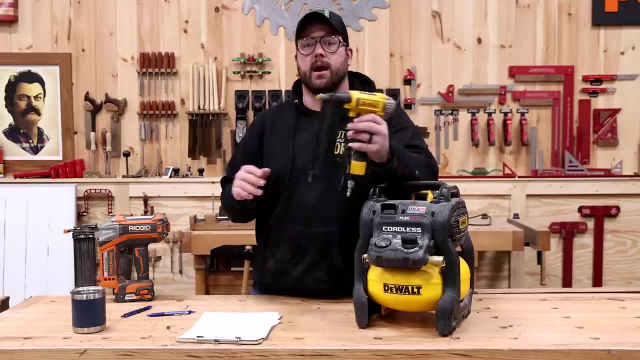 which then opens up the realm of doing a lot more. One of these 18-gauge brad nailers from Porter Cable only costs about $90. So you'd be all in at $310, which is $60 more than just this unit here. 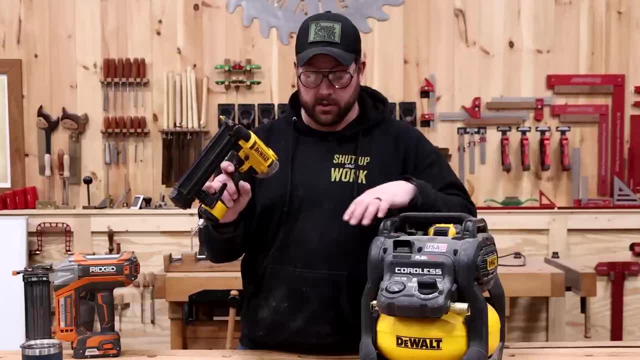 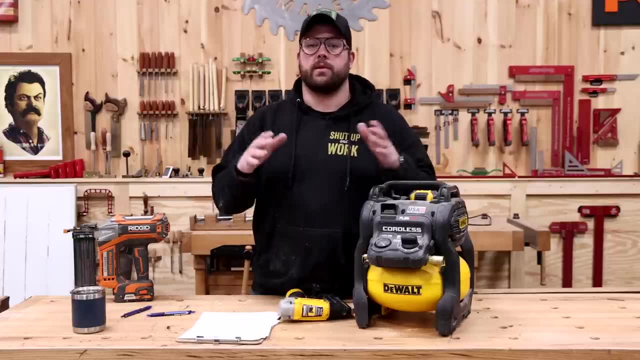 You can now shoot your 18-gauge nails, or you could purchase a 23-gauge pit nailer, which is anywhere from $100 to $200, depending on the brand, And now you can shoot 23 and 18-gauge. 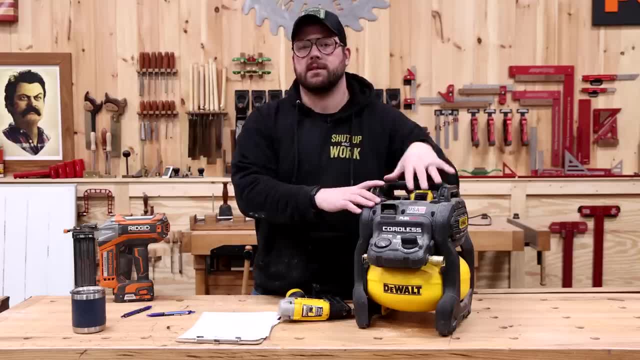 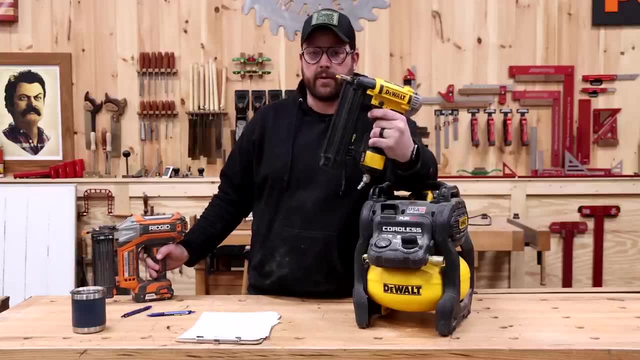 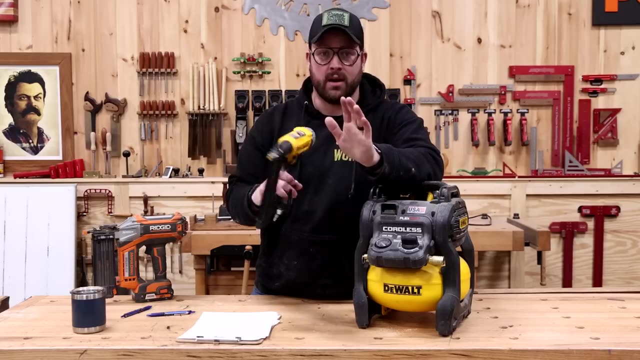 You can even step it up to 16 or 15.. You could pretty much use this thing as flexibly as you would use this Now. I will say: from a gun to a gun standpoint: you get a much more favorable tip on this. You get better penetration. in my experience, This tool is so much lighter. 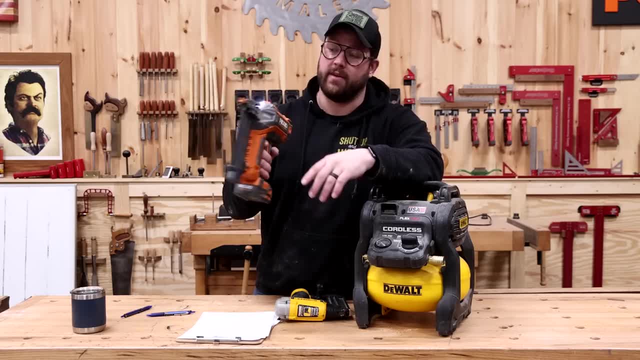 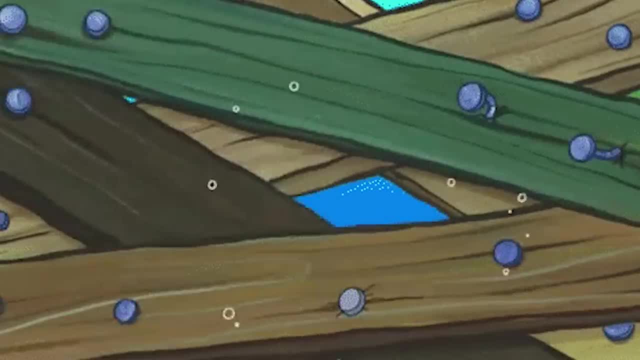 nicer to use than the battery-powered ones. These things are heavy. They've got a huge nose on them. They take a ton out of you if you're putting a bunch of nails into something, especially if you're doing like trim or if you're doing an on-site installation. It's just that heft gets. 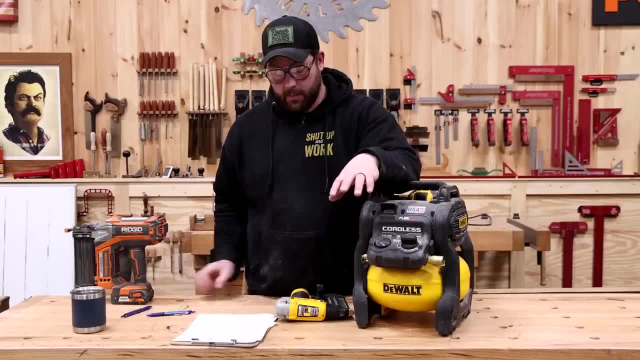 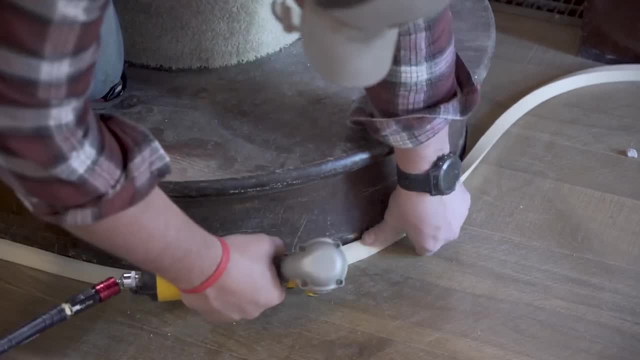 to be a huge pain in the butt, And if you're standing on a ladder it just sucks. You're better off, in my opinion, grabbing the lighter tool that you can use in and out of the shop with one of these cordless compressors Getting into the battery platform. 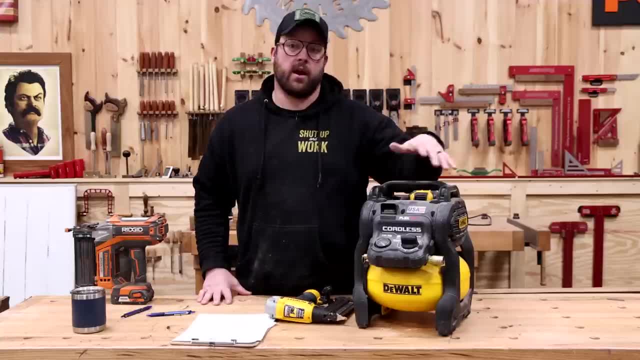 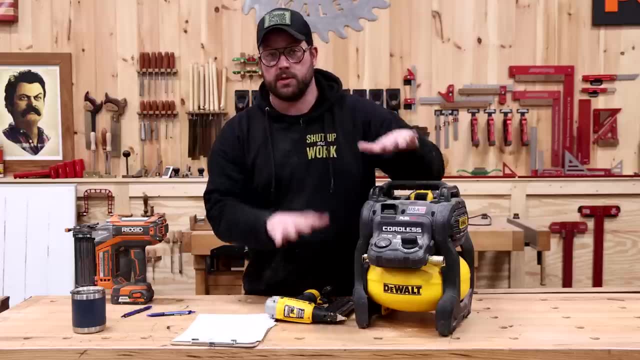 you know, the DeWalt makes a phenomenal product. I'm a huge fan. I've got a lot of their batteries, so investing in their batteries doesn't really matter as much to me. But I would definitely get into the more utilitarian tool for the shop and out of the shop than I would into one of these. 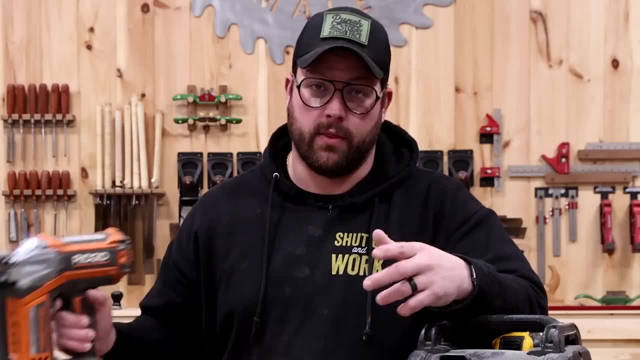 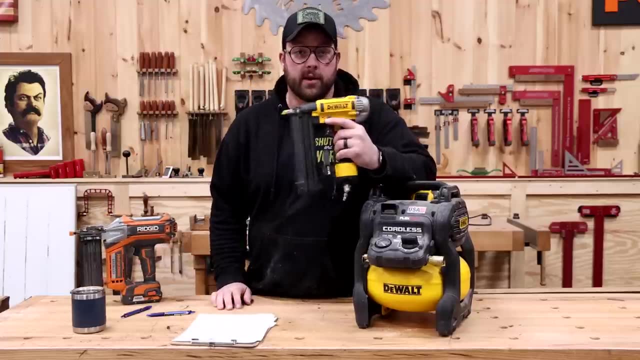 big-ass SOBs that basically only does one thing. I will say this: can only shoot one nail at a time With the compressor. you can get into one of these guns which has something called bump mode where you can just bang nails, in which goes. 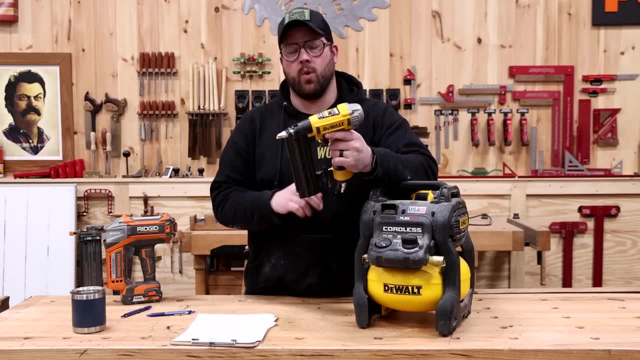 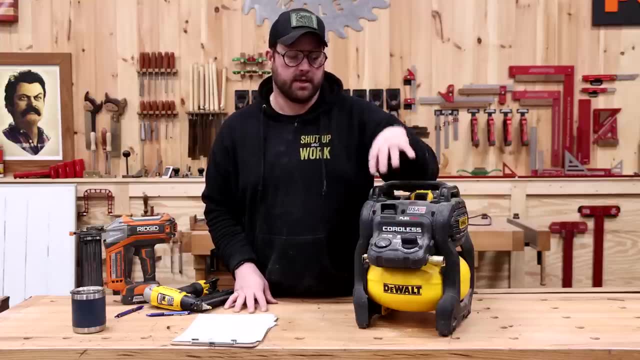 super fast, depending on the application, as well as way, way, way, way more fun to use. Lastly, if you need something to say, blow off some of your materials on a job site, the compressor comes in great handy. We've used this little guy to do a myriad of things. We have. 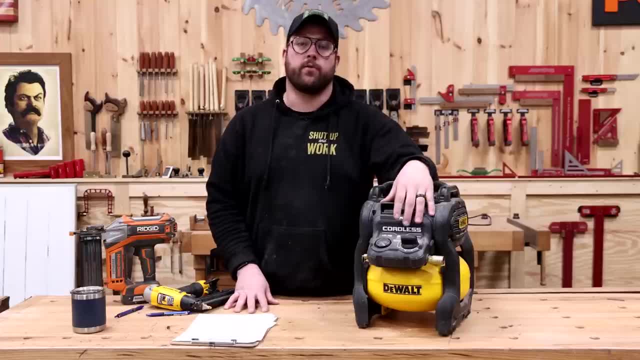 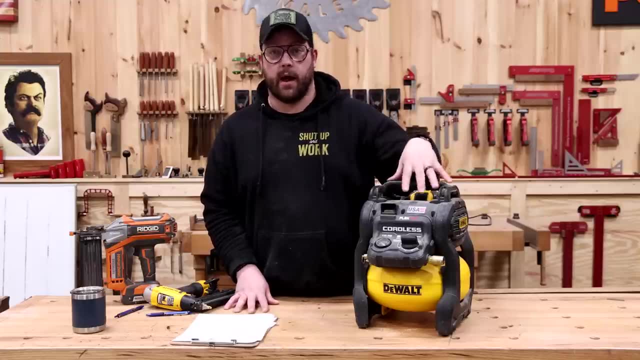 our air-based tools that we will sometimes use on a job site. If we're in a part of the shop that we don't have air run to, we bust this sucker out. It works awesome. More or less, we find ourselves grabbing this sucker a lot more than we would a cordless tool like this. So if you're going to, 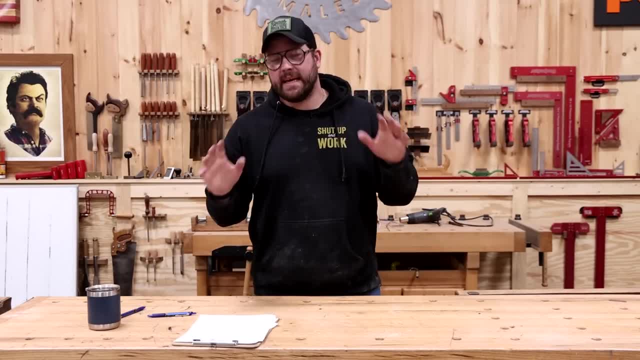 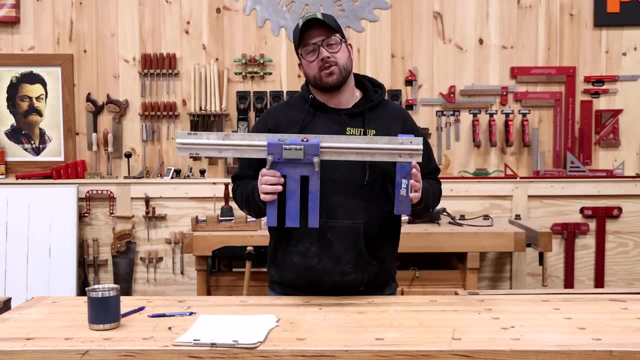 use a tool like this, it can only do one thing. So before we finish the top five, we did have a couple honorable mention tools, starting with this. If you don't know what this is, this is Craig's Circular Saw Track Guide, And I don't even know what this sucker costs anymore, but I bought 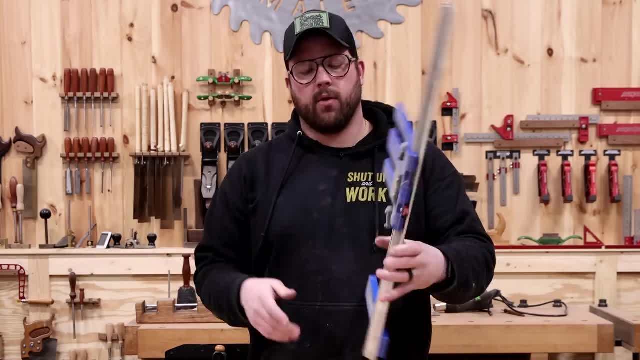 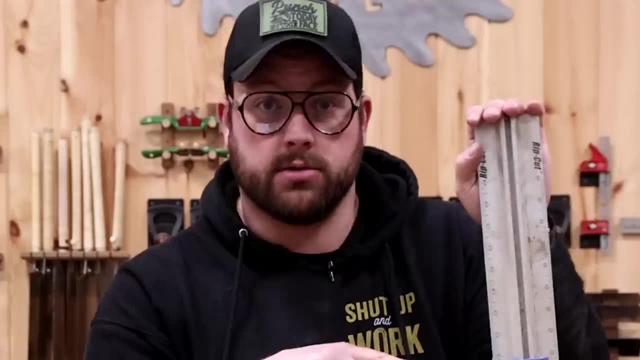 it, thinking it was going to be just like having a track saw in my shop And more or less I've come to the conclusion that any of these gimmicky track saw, hookup adjustment things are all junk. Don't buy them. You're better off making a track saw guide. 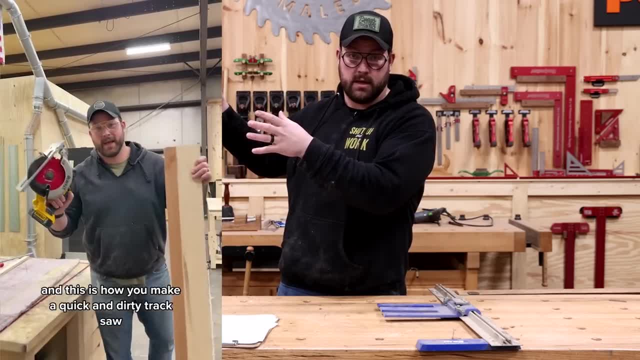 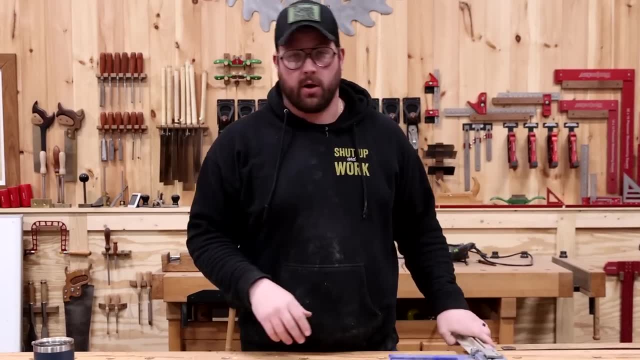 like I did in this TikTok video and using that to cut down your sheet goods. if you're looking for something that's going to give you that straight line sort of track saw, cut, Don't waste your money on this junk. The second tool that I don't think a beginner should waste their money on is this. 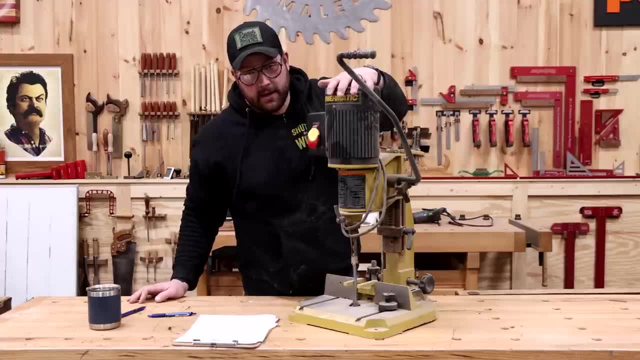 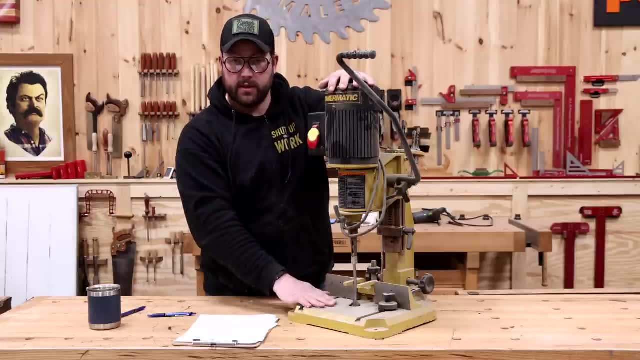 sucker. And no, that's not a drill press. This is a hollow chisel mortiser. When I started to step up my woodworking game and I wanted to get into doing mortise and tenon joinery, I really thought that this tool would come in handy, but it turns out it's just more of a cheap tool, So it's. 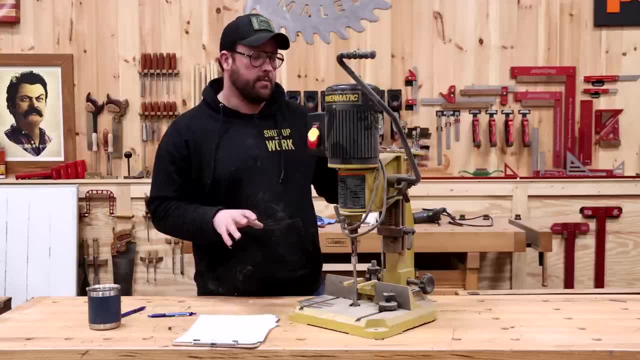 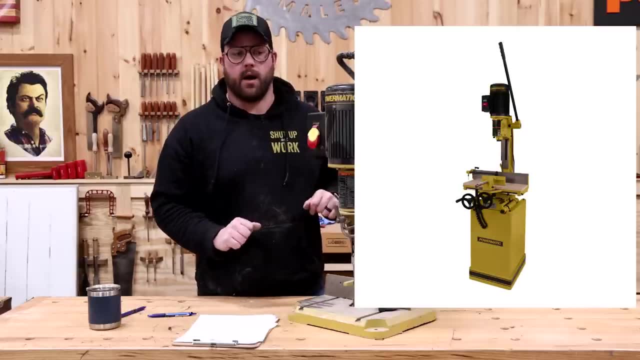 more of a pain in the butt than it is anything else. It costs a bunch of money. The bits are really hard to keep sharp. It has a lot of little cues and quirks and whatnot to it And they're great tools. if they're a floor model, I really don't like the benchtop model Once you get into. 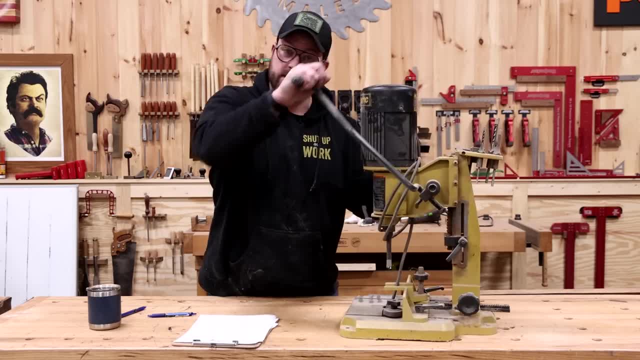 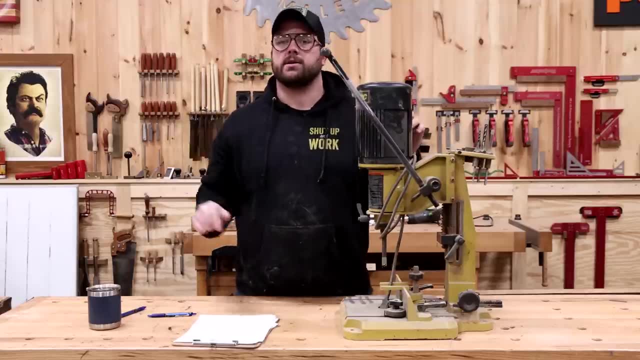 any bigger materials. this thing is racking all over the place as you're putting pressure on it and whatnot. You'd have to fix it to a table anyway If you want to get into doing mortise and tenon joinery. there's way easier ways with routers, dominoes or a floor model like this. 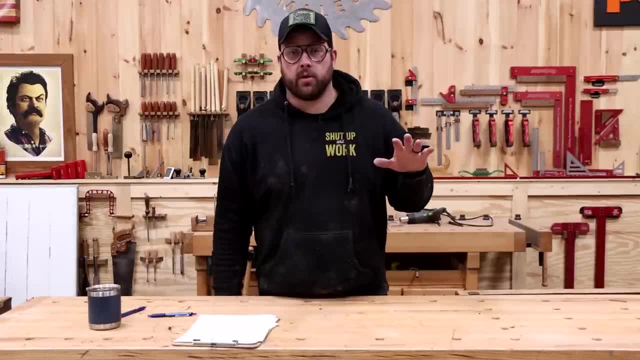 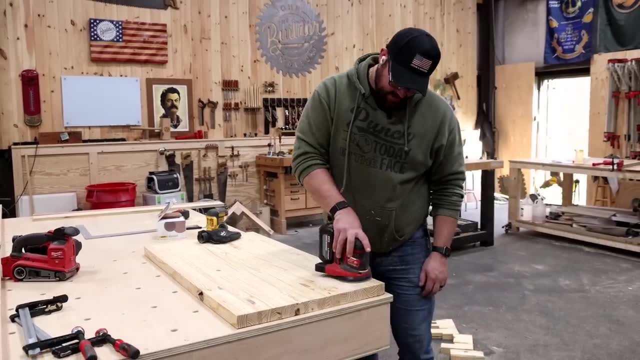 that you can buy used on Craigslist, Do not recommend for the beginner. Third honorable mention tool on my list is going to be any, and I mean any- cordless palm sander. I've used a bunch of the big brands, including the Festool, which is awesome, but it's still not. 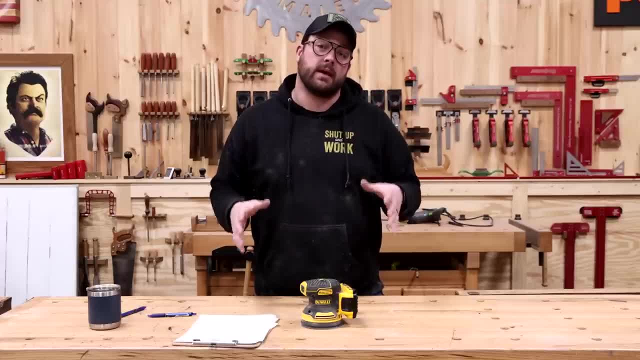 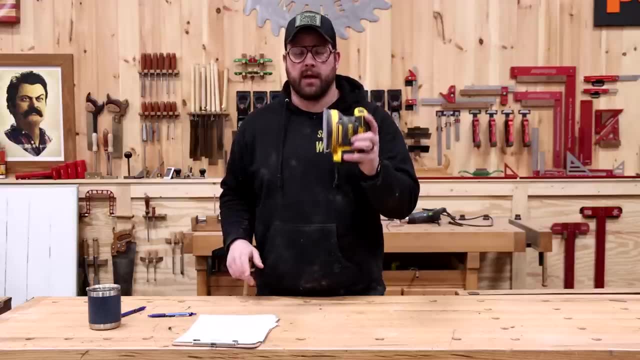 worth the money. If you're a woodworker and if you're sanding, you're probably going to be in a shop near a plug even when you're on site, Unless you're working outdoors in the middle of the woods. I still don't recommend this. You're better off plugging a sander into a. 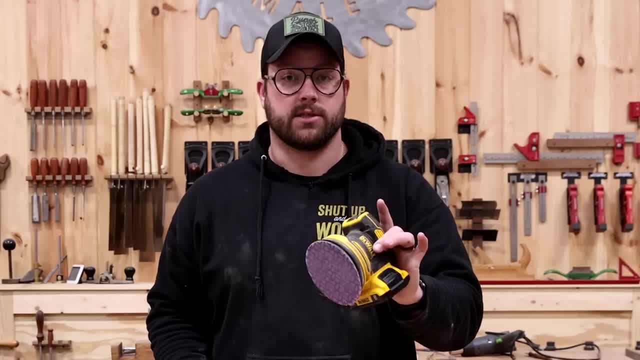 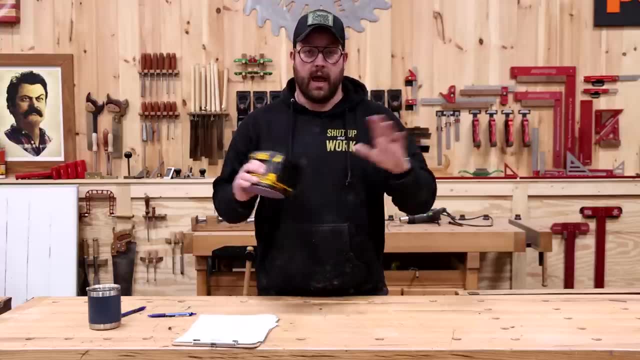 generator or something else. These have terrible ergonomics. The dust collection sucks, The power is terrible. I just really don't see the benefit of spending more money to get a cordless tool like this in any regards. Sorry to all you brands out there that are investing heavily in it. 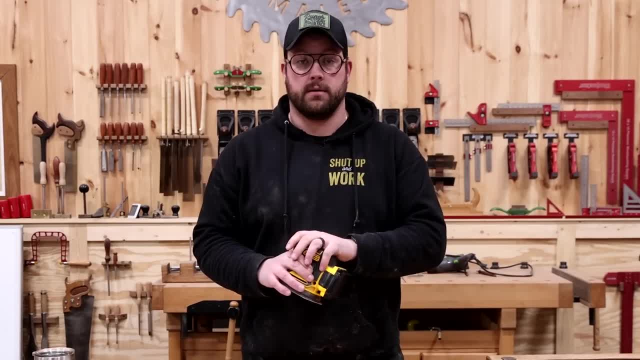 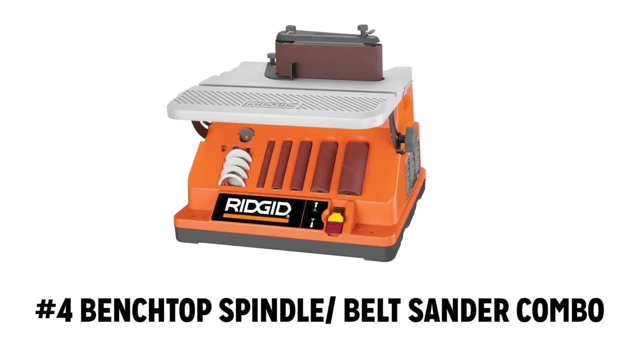 but you're never going to be able to beat the plug-in palm sander, so don't waste your money. Number four: benchtop spindle belt sander combo, specifically from RIDGID. Now, I don't know who else makes these, but when I was getting started they were all over the 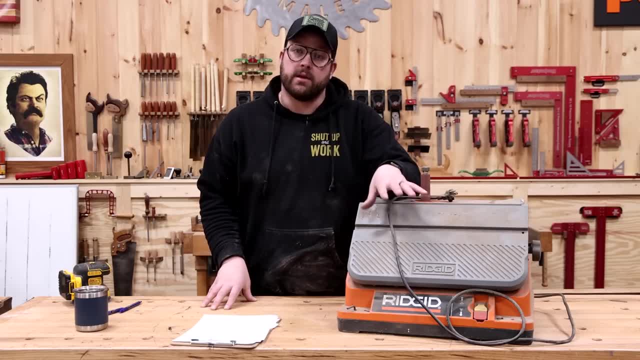 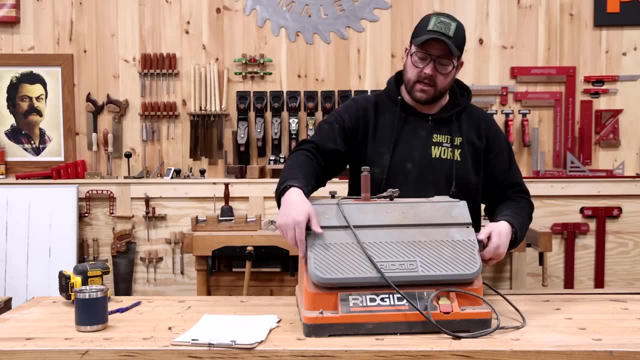 internet and I thought they were awesome. I thought it was super cool. I really, really wanted them. I have FOMO, just like you guys. I want all the cool tools that I see on the internet, but the problem with this sucker is I've broken three or four of them. One- it really just doesn't. 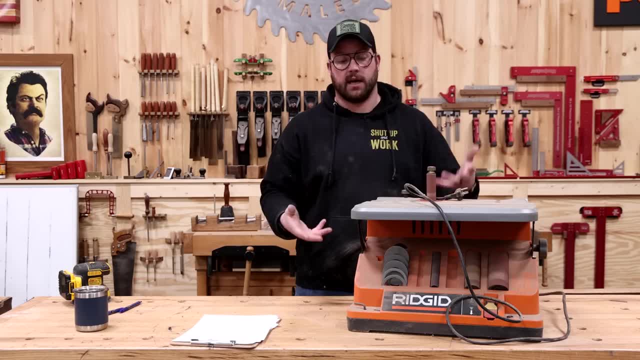 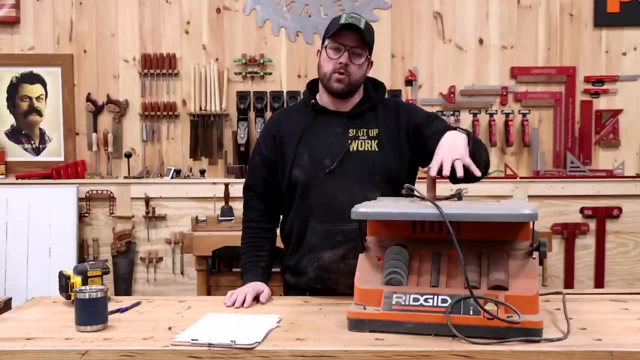 get used enough. It literally sits on the bench and collects dust. As you can see, this sucker is just dusty as hell and it's just not that necessary to spend your money on when you're getting started. You can get accessories for other tools in your shop, like your drill press. 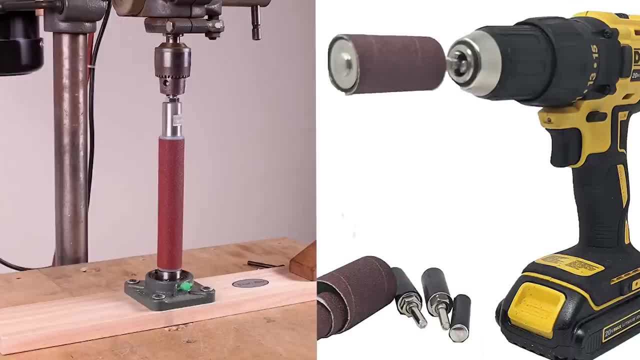 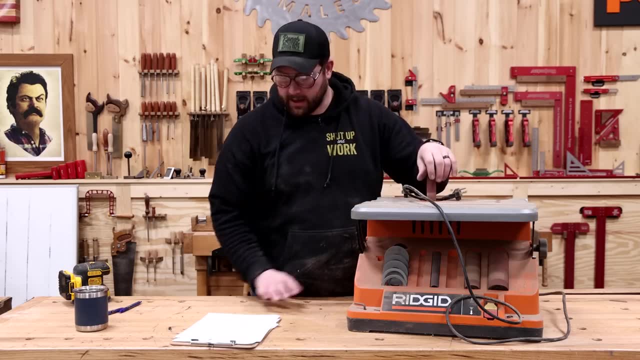 or your handheld drill to do curves way easier. They make handheld sanders that do this kind of stuff. You just don't need it and it's super pricey. Last time I checked the price I was too dumb to write it down, so I'll put it up on the screen. 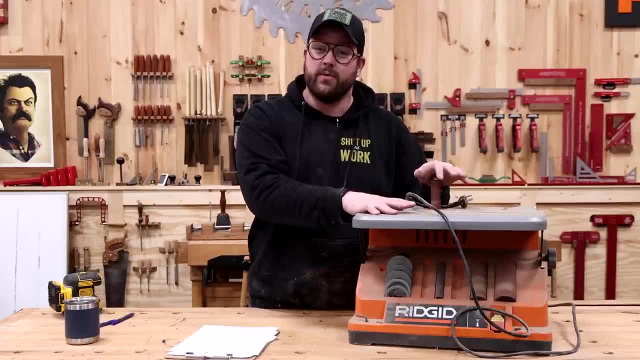 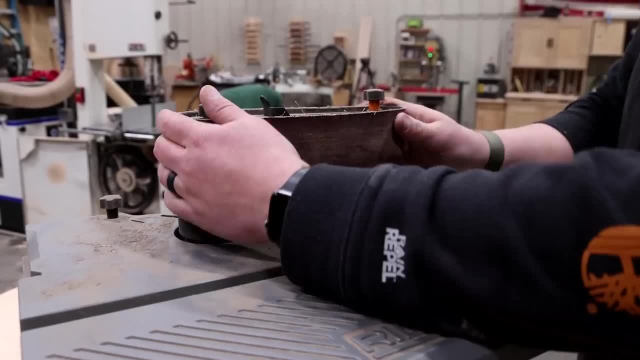 right here, but you can invest in a lot of other stuff before you get into this, or even build something yourself to do the same thing. Not worth the money. Don't buy it if you're just getting started. Like I said, with the hollow chisel mortiser we've used my floor model spindle sander. 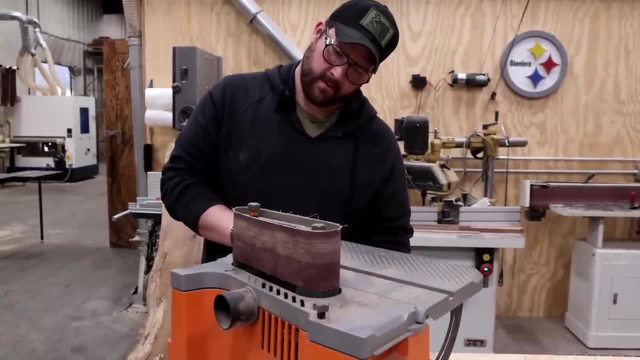 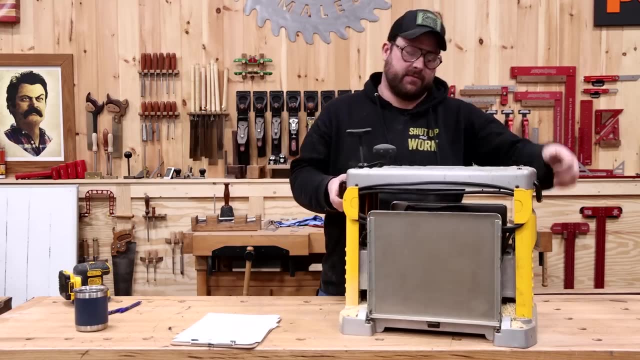 way more than we ever used this thing, and I've had that way shorter than I've had this. This sucker's been on a shelf for a long time and it's been a long time since I've used this thing. This sucker's been on a shelf for nine years. And last but certainly not least, rounding out my top five, 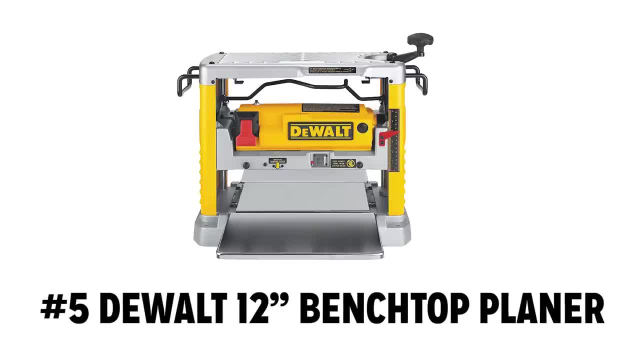 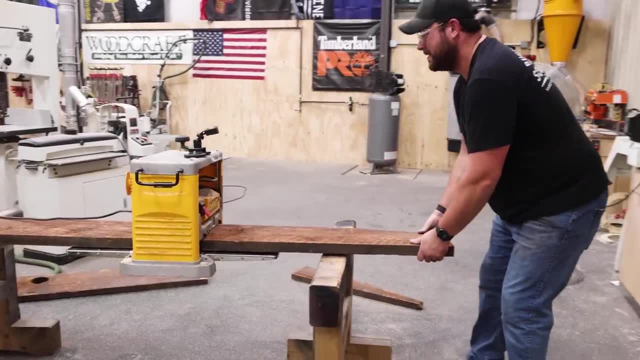 is going to be the DeWalt 12-inch benchtop planer. I've put this old girl through her paces for a long, long time and I don't actually necessarily dislike this tool. It's fine, It's a good entry. 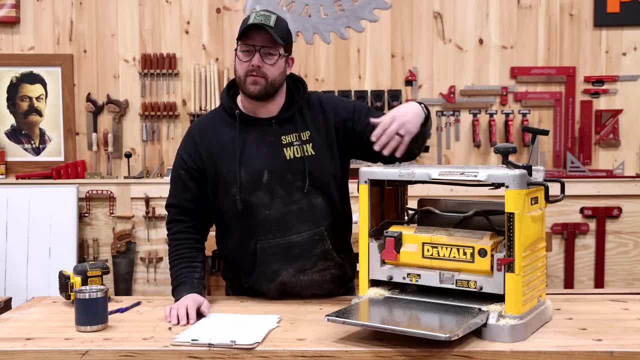 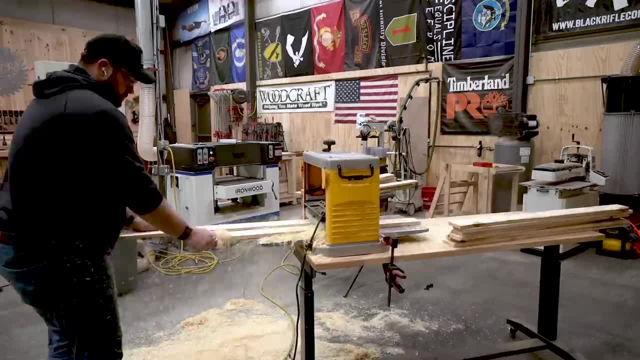 this tool, But some of the problems that I've had over the years have been: one doesn't have a ton of power. Don't care if you're in a 20-volt outlet. I constantly pop this little button here and blow. 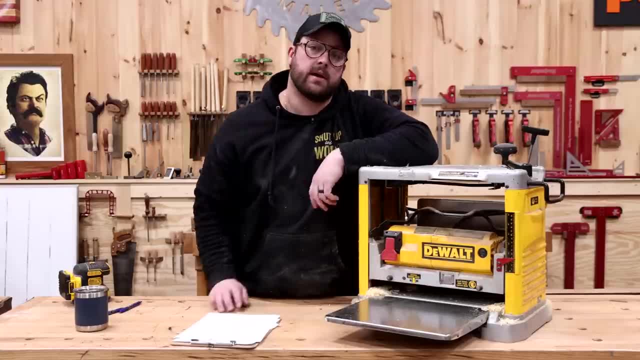 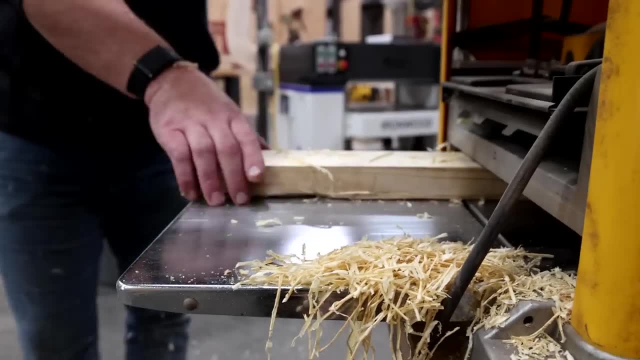 it out. If you remember our pallet video where I only used this and our job site table saw to build a table, I was blowing this thing out left and right, just running straight pine through. it Doesn't have a ton of oomph or balls as I would typically say. It's also 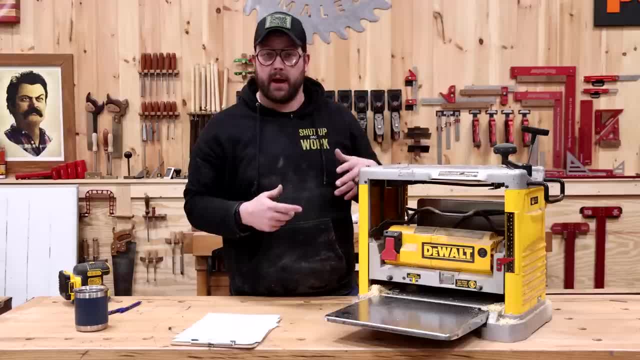 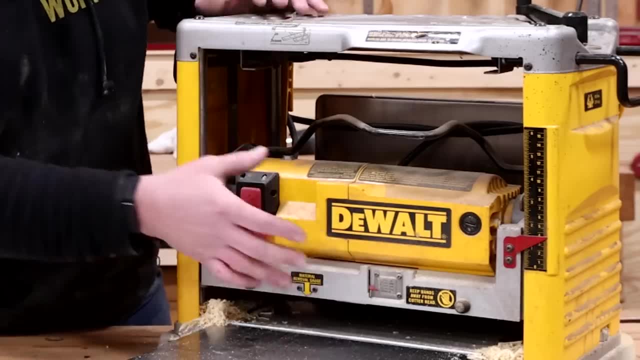 super, super heavy, 80 pounds. They claim that you should have two people using it. The problem isn't that it's heavy. The problem is it's top heavy. A lot of that weight's in here, So as you're putting stuff through it, it tends to want to tip over, And I've had that issue for a long. 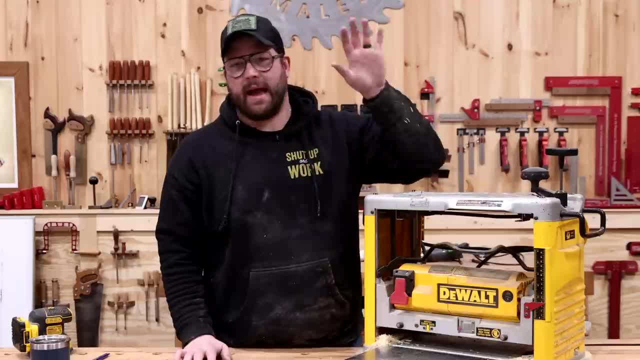 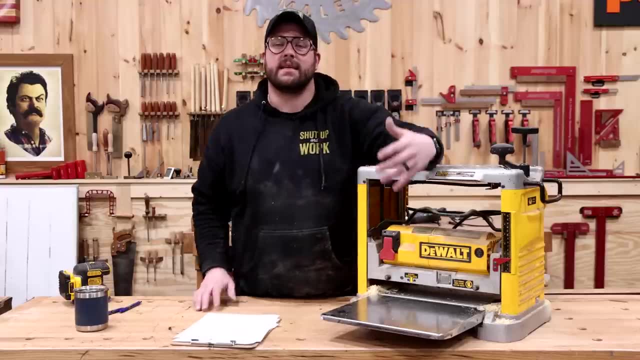 time You have to fix it to something. Even then you're going to feel like I had constant problems with tipping the whole thing over. And it's not very wide either, So the base of it is not very stable. The dust collection on it is decent, The tooling on it is decent, But if you're not familiar, 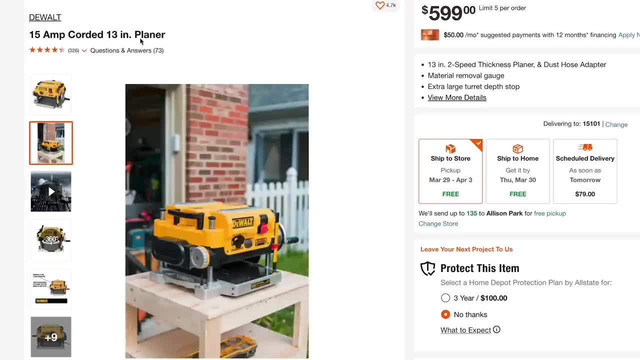 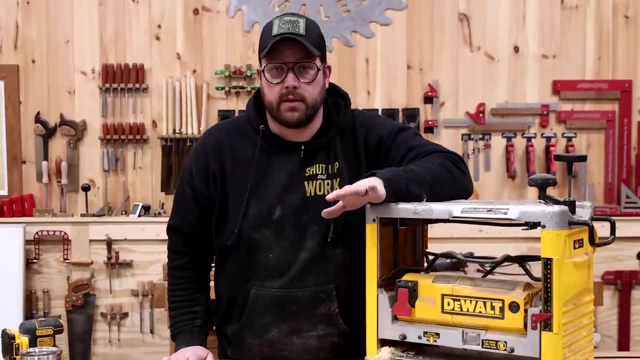 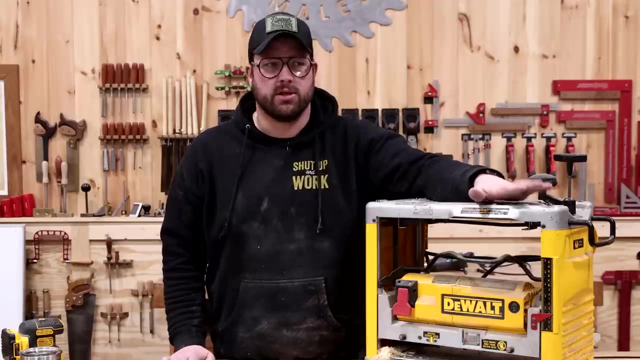 for a hundred bucks more you can get into the DeWalt 13-inch benchtop that I've used in a few of my friends' shop And it is night and day difference. You're getting much closer to a professional feel on that tool than you are with this lunchbox. You're getting another inch to. 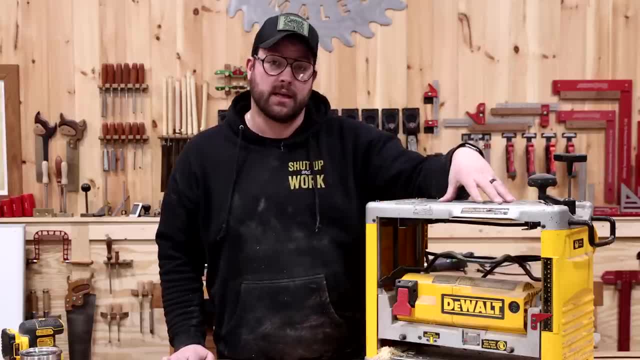 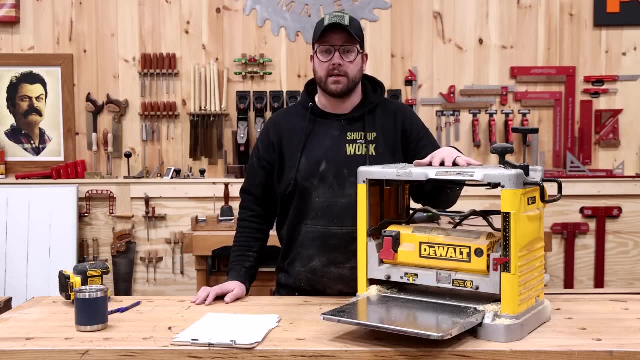 I think almost an inch and a half of width on your boards and capacity. I'm going to pump those numbers out. Those are rookie numbers. They make Shelix heads for it that you could put in, which are carbide inserted heads. The dust collection is. 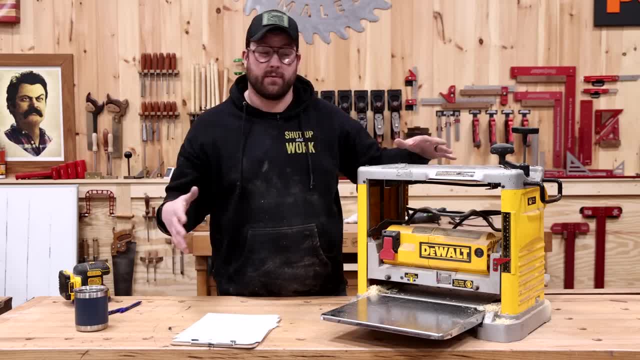 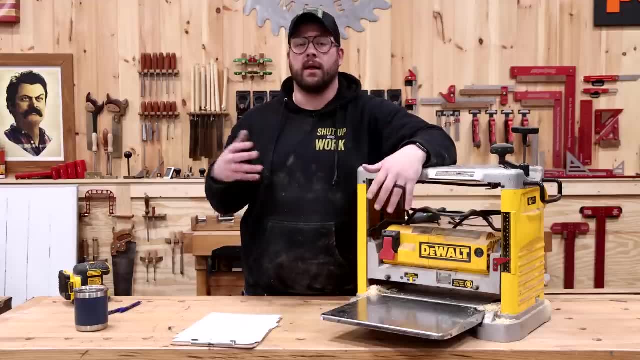 10 times better than it is on this. It's built wider, so the center of gravity doesn't tend to tip. There's tons of YouTubers using it for a reason And there's tons of pro shops on a smaller scale that run that tool because it's just so much better. Don't be cheap. in this regard, The 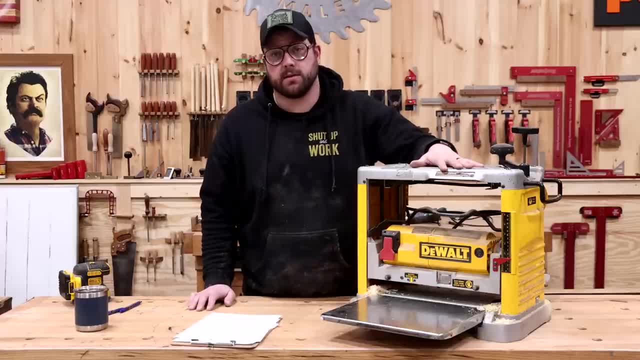 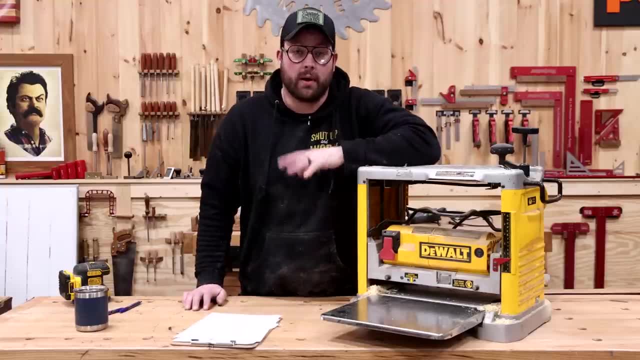 reason I don't recommend this for the beginner is because it's worth investing the extra hundred dollars. I've had more downtime just waiting for this thing's breaker to turn back on than I have with any other tool combined in my shop. So save yourself the headache. Spend an extra hundred.